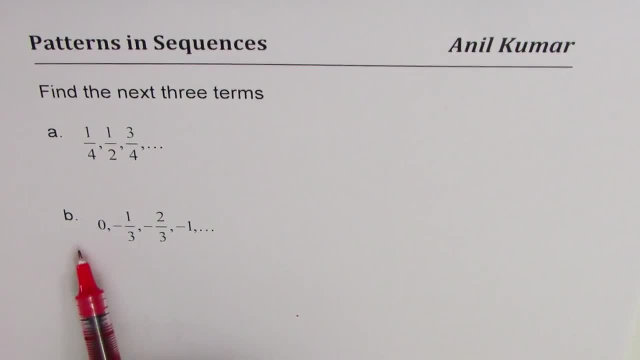 next three terms of this sequence and then we have 0 minus 1 over 3 minus 2 over 3 minus 1.. You can always pause the video, answer the question and then look into my selections. Now, in questions involving fractions, what is our strategy? 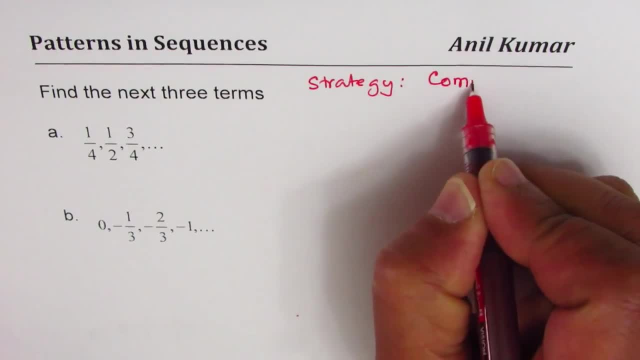 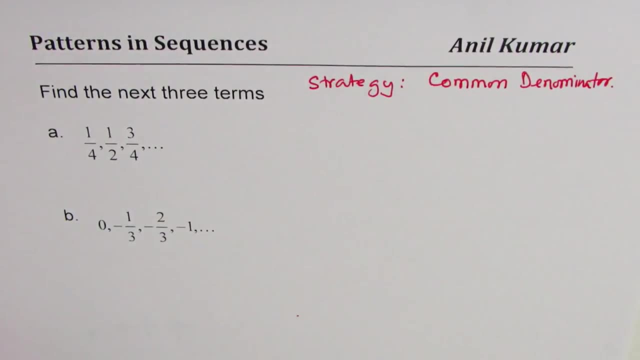 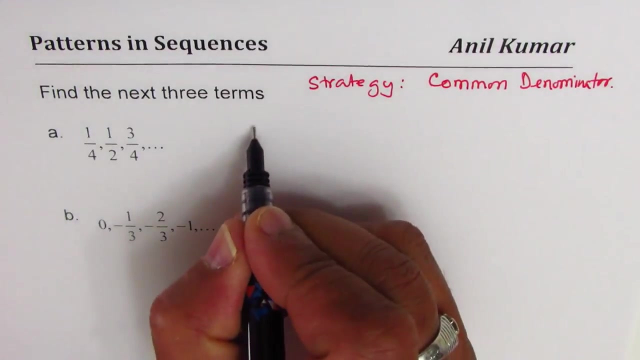 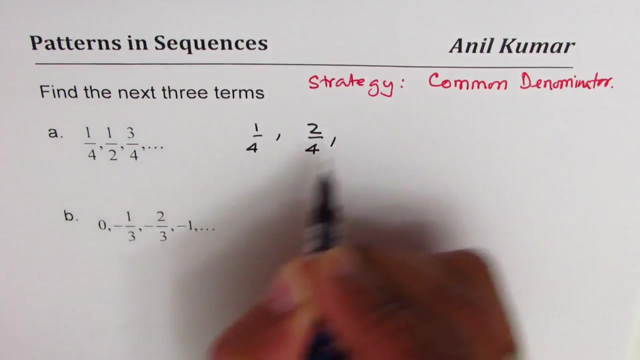 Strategy is to have a common denominator right. That is the strategy Correct. So let's rewrite the question with a common denominator. 4 could be the common denominator right, so I could write this as 1 over 4. multiplying by 2, I get 2 over 4 and this is already 4, so 3. 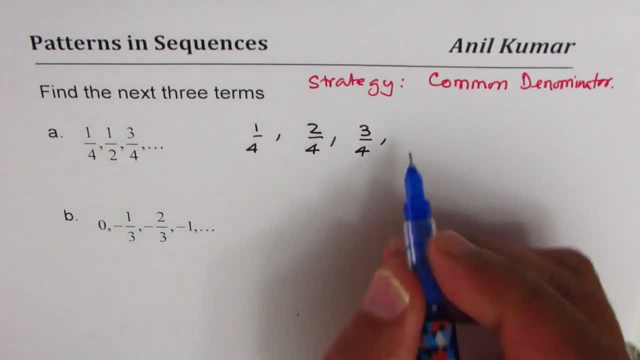 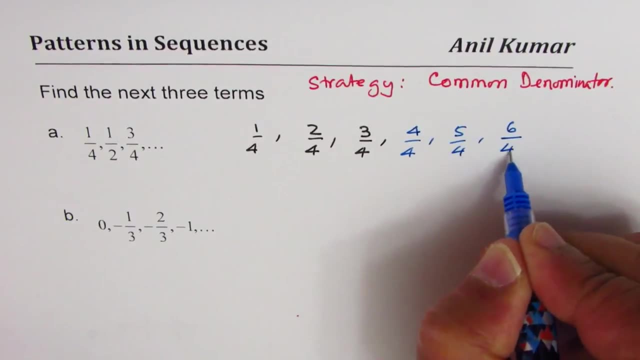 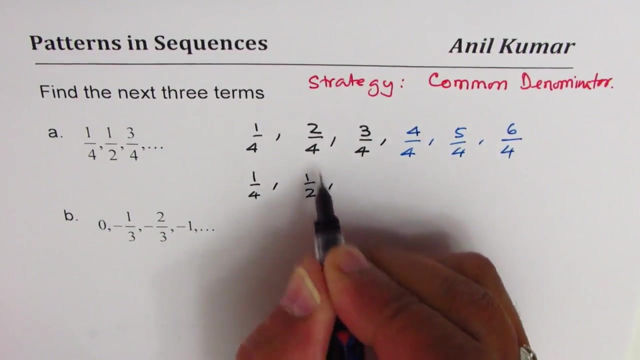 over 4. correct, so clearly we get the next three terms as 4 over 4, 5 over 4 and 6 over 4. so now I can rewrite the whole pattern as 1 over 4, 1 over 2. that is simplifying, right. 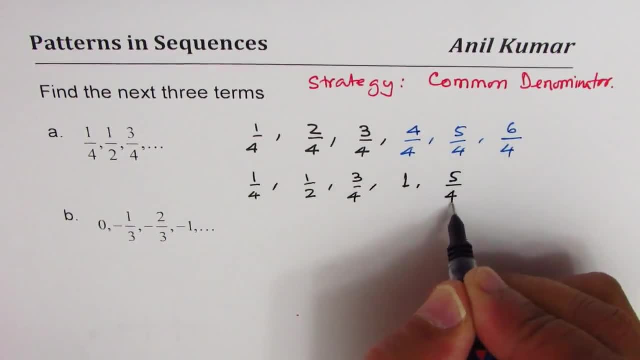 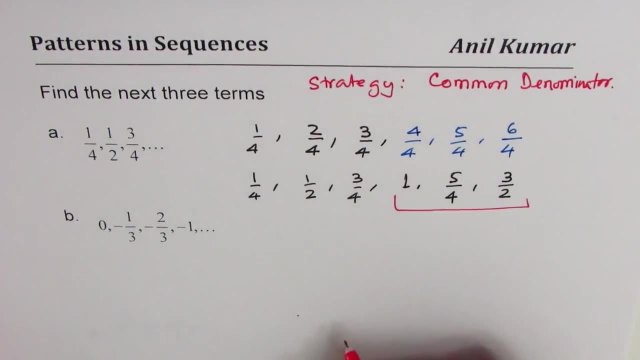 4 over 4 is 1, 5 over 4, 3 over 2, right? So the next three terms are these: Perfect, so that is how you could actually very easily Check for the patterns. Which involves fractions in a sequence, right? I'd like you to answer the next question. take your time. 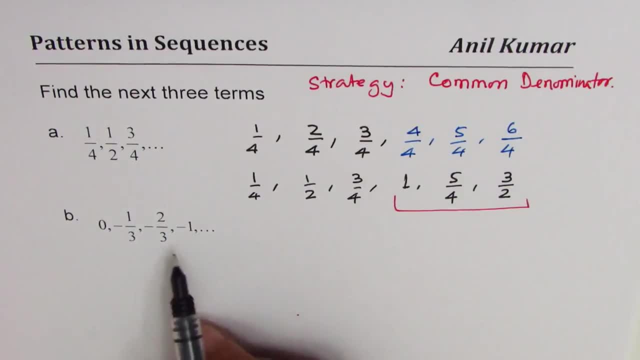 Here is my solution. Strategy is seen, will make denominators 3 for each right, so I could write this as 0 over 3 and then minus 1 over 3. We already have this as minus 2 over 3. Minus 1 could be written as minus 3 over 3, correct now? Do you see a pattern? 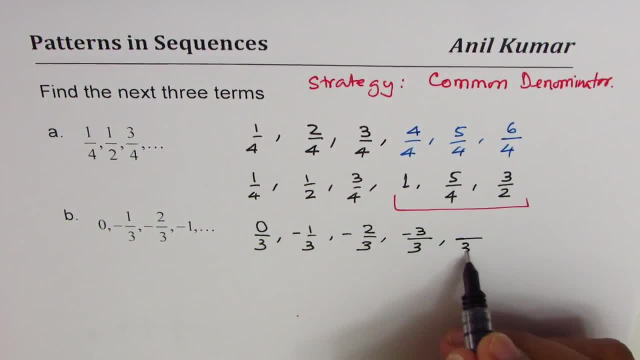 so the pattern clearly is, denominator being 3, numerator is an integer moving left right less by 1. take away 1, so minus 4 over 3, minus 5 over 3 and Minus 6 over 3, so those could be the next three terms.